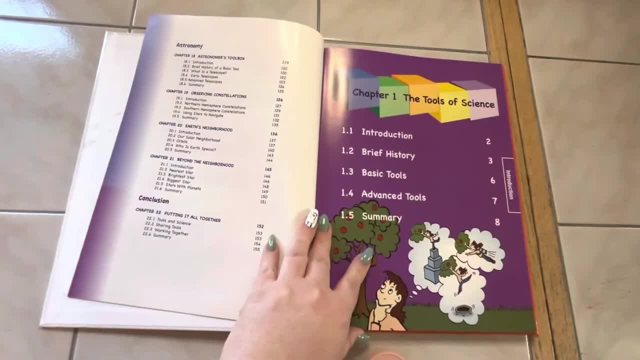 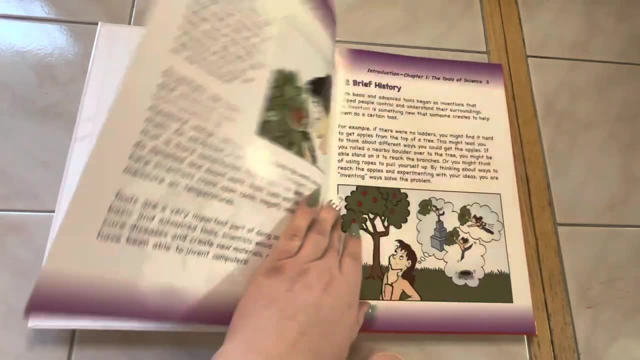 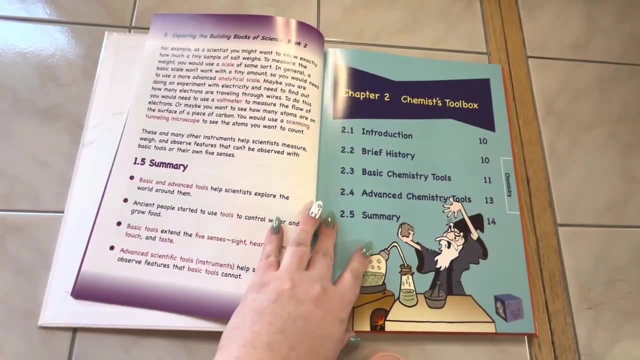 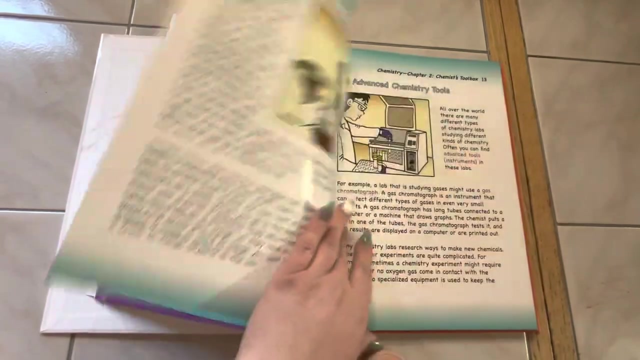 and chapter one. So they will go through, like the brief history, basic tool, advanced tools and summaries, And then in chapter two they go into the chemist's toolbox explaining, you know, a brief history, basic chemistry tools, advanced tools, the acids and bases in chapter three. 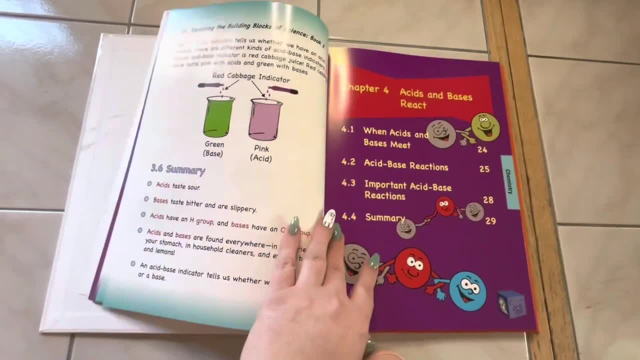 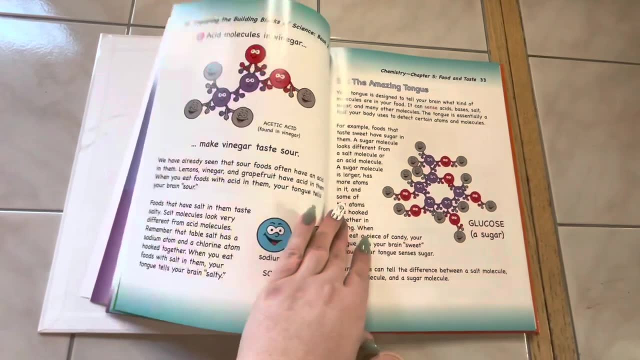 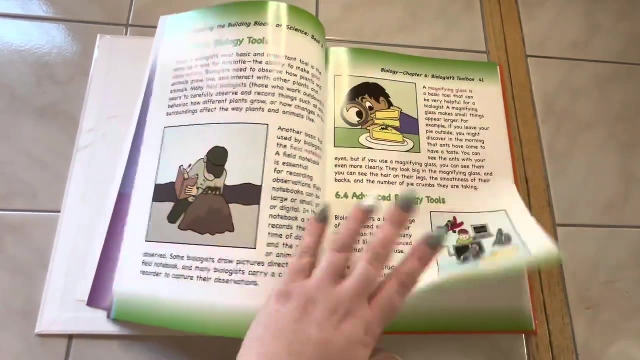 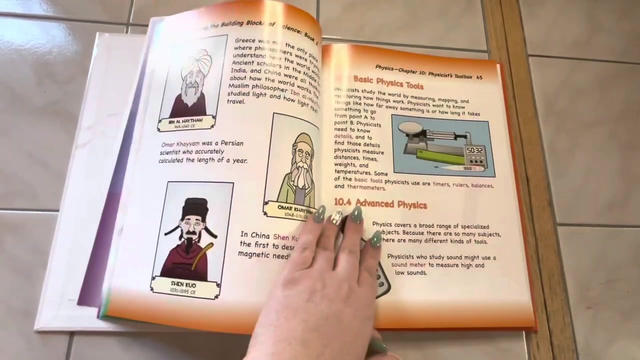 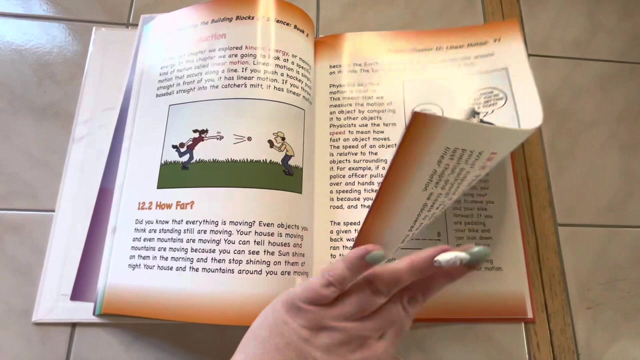 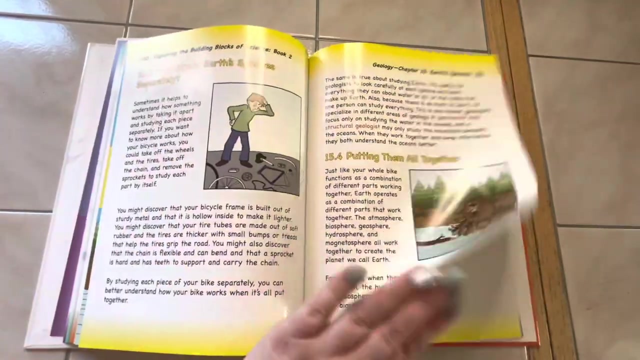 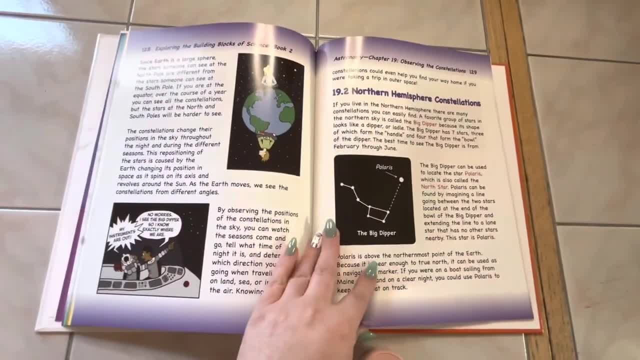 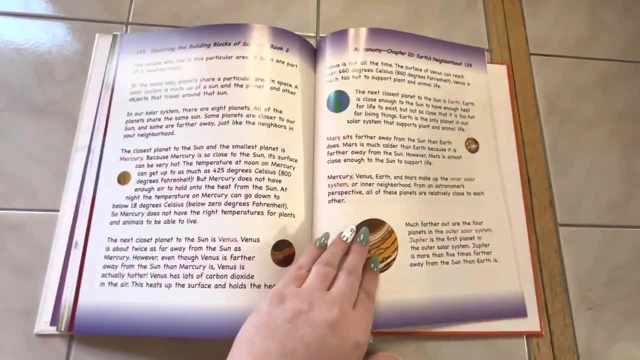 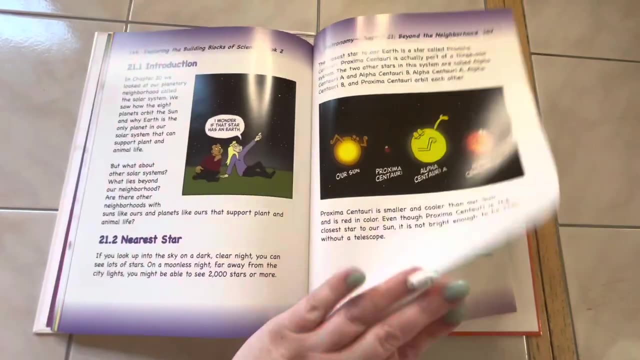 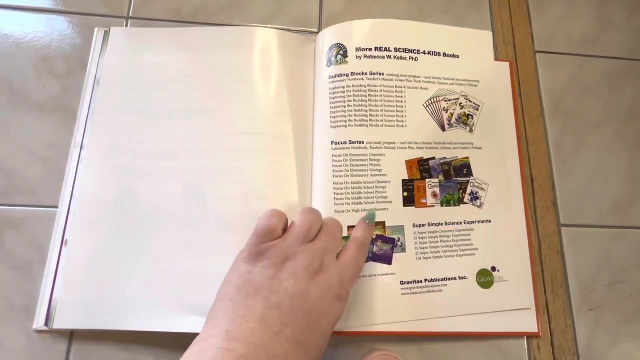 Geology And, last but not least, they go into astronomy And then here in the back they show other things they have. So they have the focus series, super simple science experiments and then, of course, the building blocks of science series. 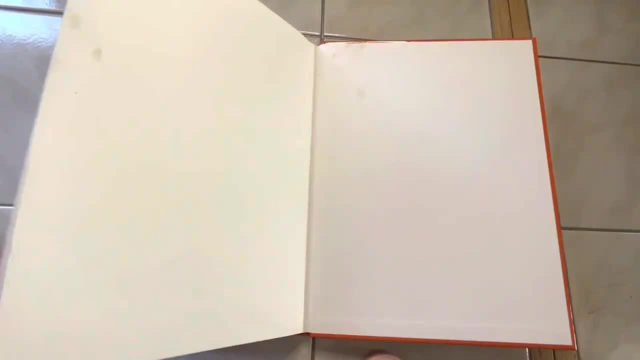 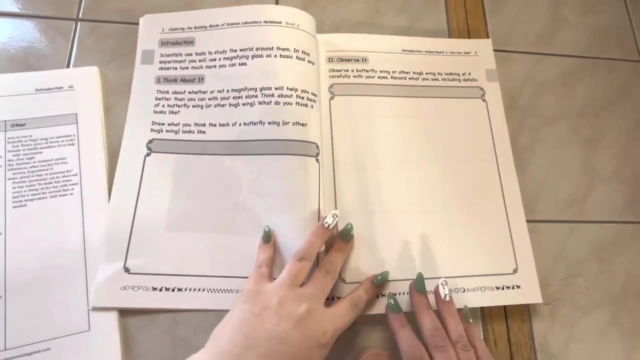 And that is everything there. So it just literally ends the book with a little ad at the end. So this here is the laboratory notebook. We do not fill these out because of we just don't. A lot of the times my daughter and I do everything verbally. 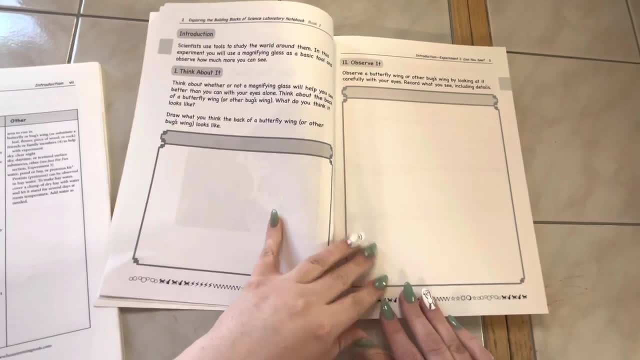 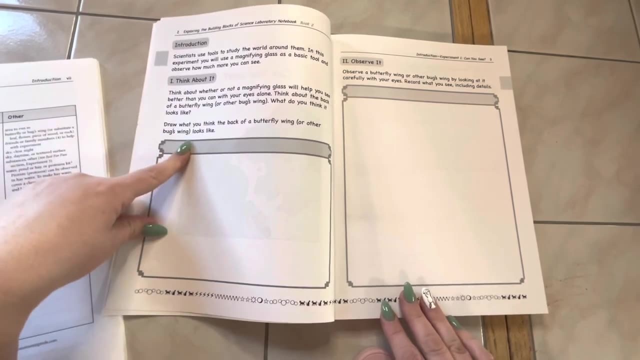 Sometimes we skip some of the pieces and we just do the actual experiment. So here it'll tell you the introduction, It'll tell you to think about it and it'll read that to you, And then it'll say: draw what you think: the back of a butterfly's wing. 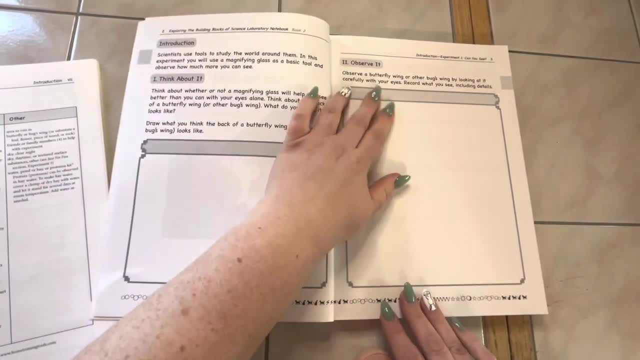 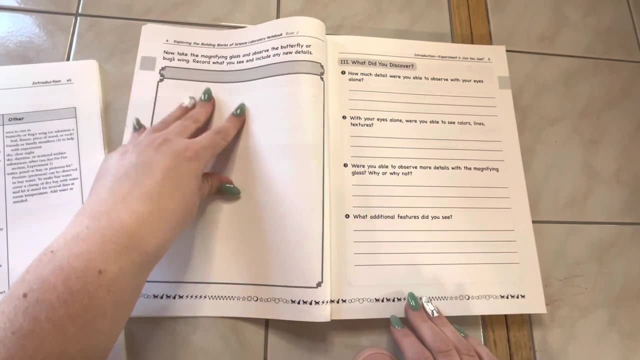 or other bugs would look like. Then there's the observe: Observe a butterfly wing by looking at it, Record what you see. Take the myofascial gas and observe the butterfly or bug's wing. Record what you see and include any new details. 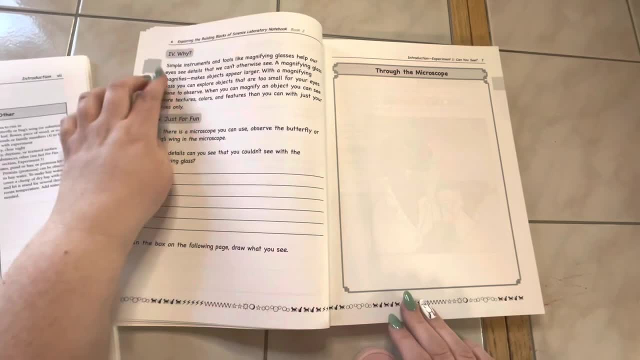 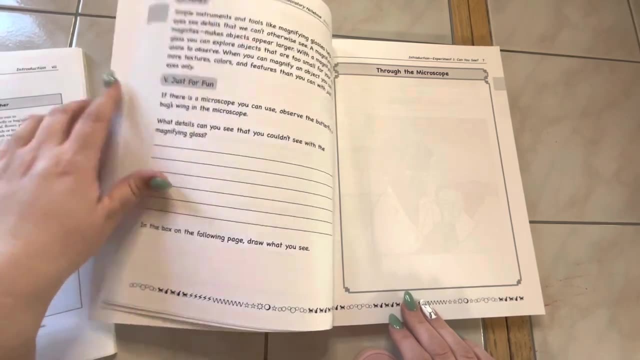 What did you discover? Why? And then, just for fun, if there's a microscope you can use, observe the butterfly or wings in the microscope. So you don't have to do this section. Honestly, we don't do all of this. 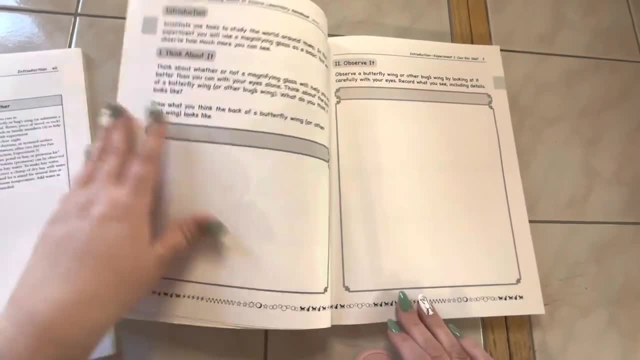 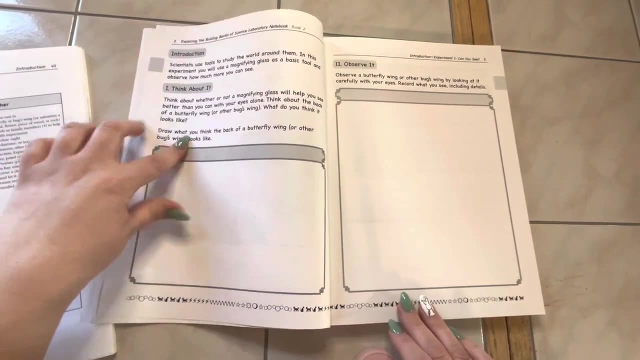 Anyways, a lot of the times I know for this specific experiment. when we did this I just had I read the introduction, I read the think about it. I skipped the draw part and I said I had her while we were looking at a butterfly wing. 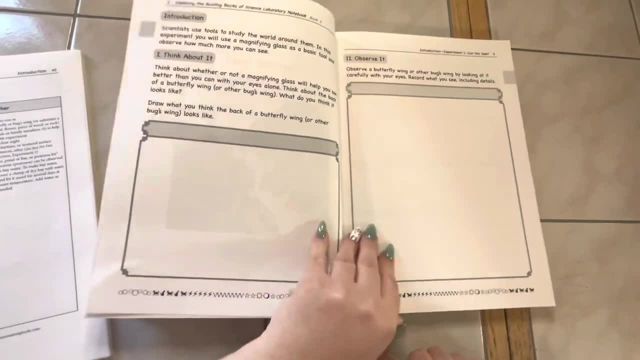 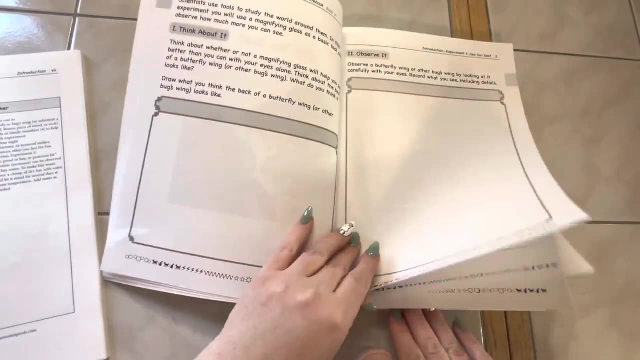 tell me what she could see and how it was working. Now, all of these pages are very similar in this nature. It just is the experiments for your child. It goes through the information you would need to do any of the experiments in here. 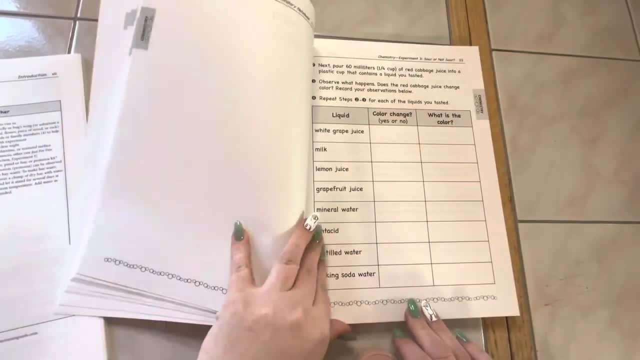 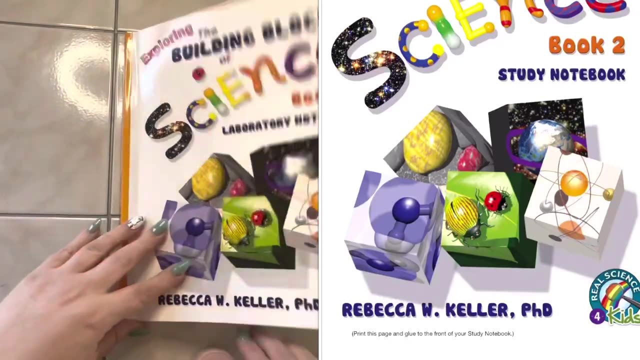 I just end up leaving a lot of it blank because we talk about it out loud and we don't actually write it down in the book, which I think is perfectly fine. I do have her do the student study notebook, which is, I think, fun and engaging for her. 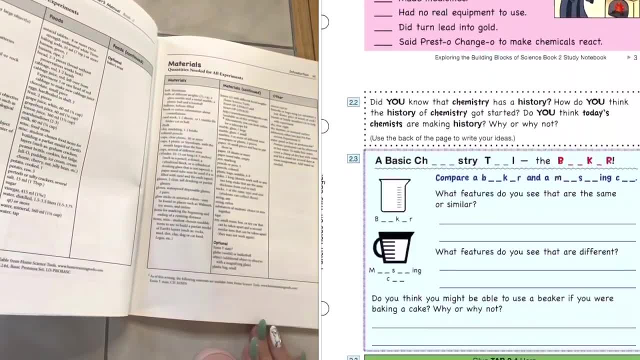 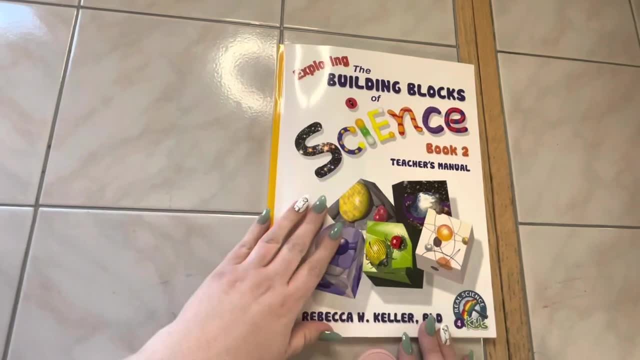 I will put a screenshot in here for you guys to take a look at the student notebook in a minute here and you'll scroll through that. and I'll just scroll through that so you can take a quick glance. And then this is the teacher's notebook for teacher's manual for building blocks of science. 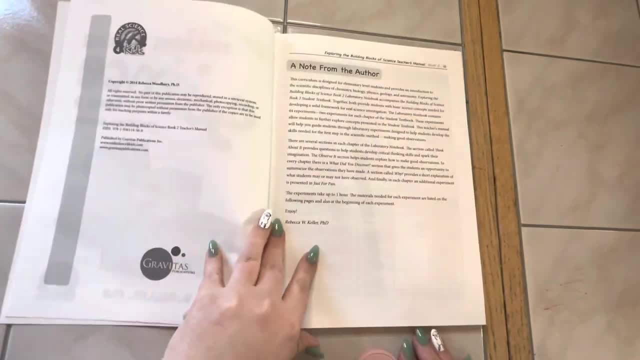 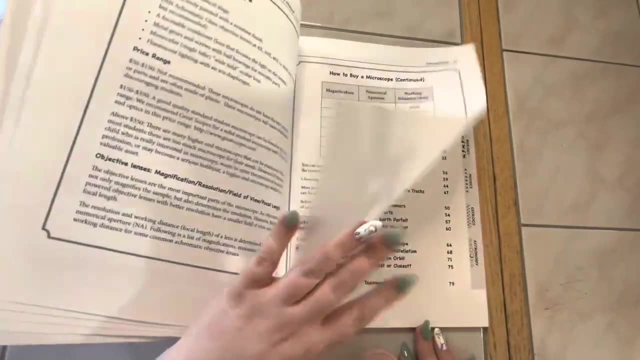 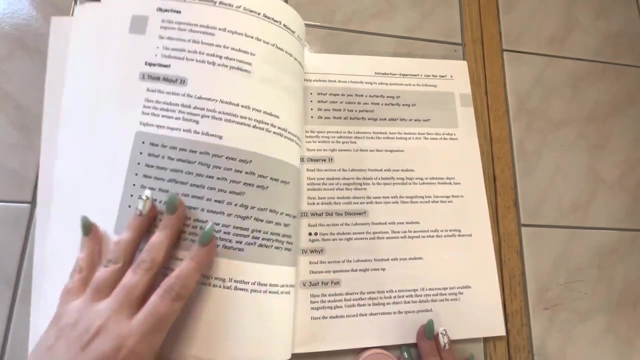 I, I love that it has the note from the author, it has the materials you would need for each experiment, And then it tells you how to buy a microscope, which I think is really cool. And then, of course, we can pop over here to this same butterfly one. 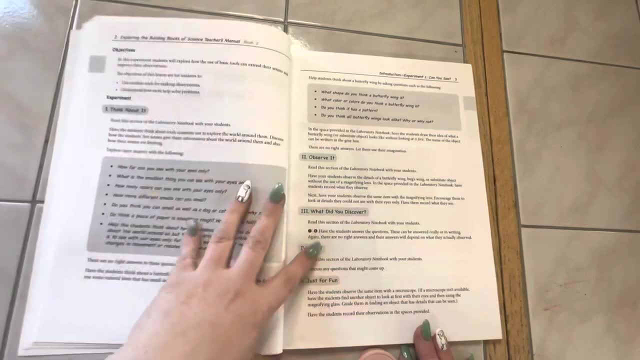 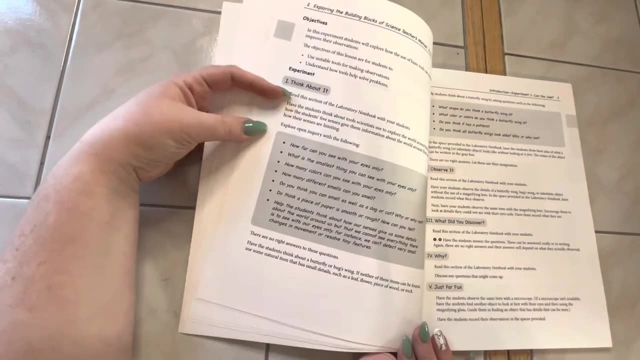 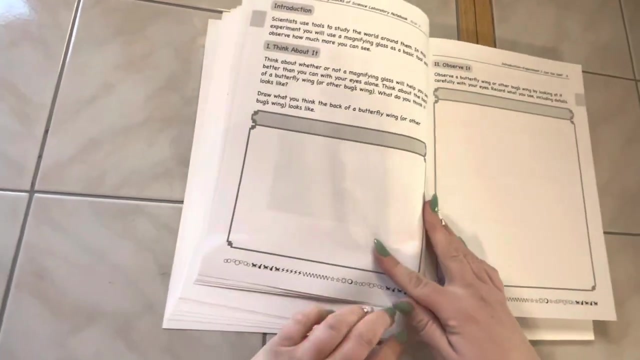 where it shows you what you would need. Then it also goes through here and tells you what the objective is, So what they'll be learning, And then it says to read the section in the notebook. so that would have been the think about it section in here of: can you see the introduction and think? 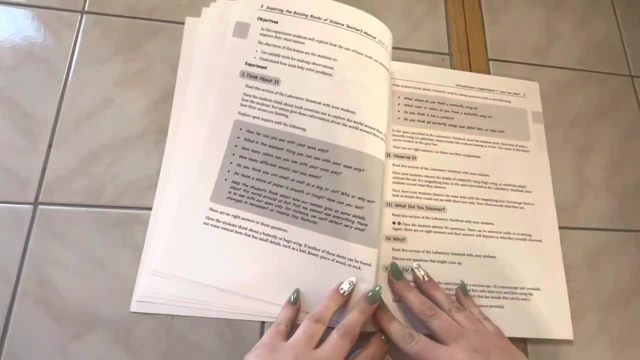 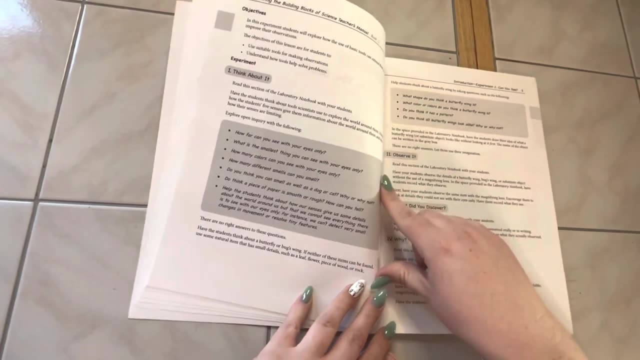 about it. so you would read that to your child and then, of course, when it says, explore open inquire with the following: how can far can you see with your eyes? only what is the smallest thing you can see? it explains to help the child by asking these questions. read the section in the lab. 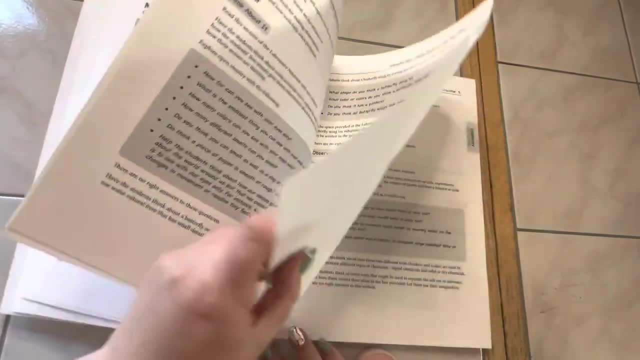 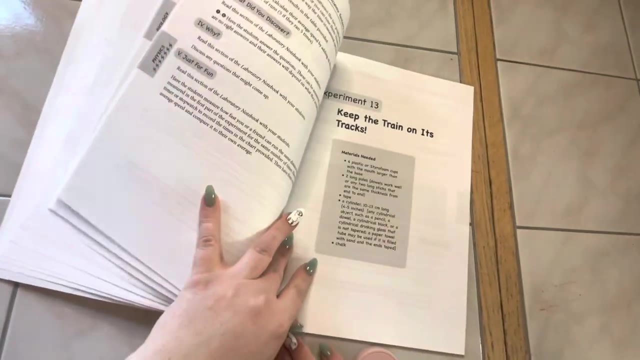 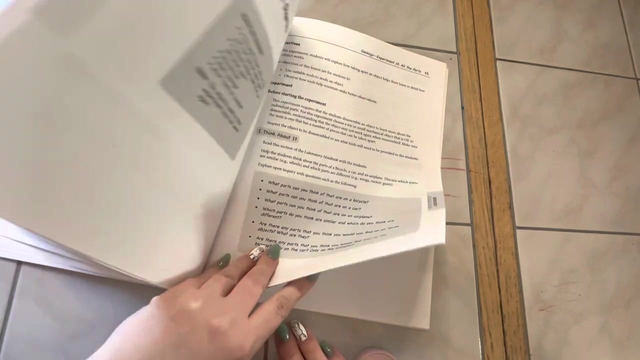 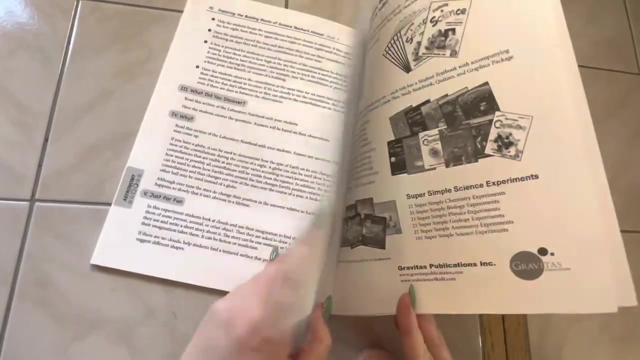 notebook, have your student observe and detail so it tells you what to do. and then it does that for all these. so chemistry, biology, physics, geology and astronomy. my son is here. he just woke up from a nap, so he is back there shattering away. um, my biggest complaint, which probably is a small. 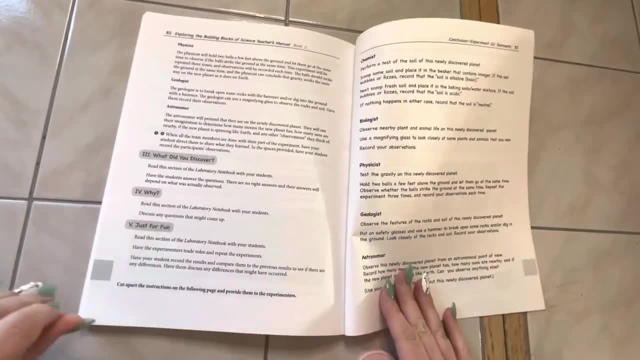 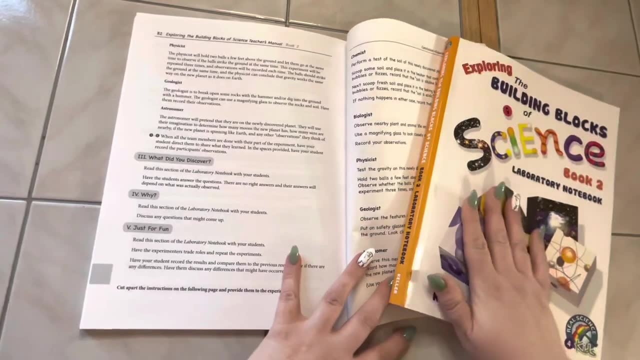 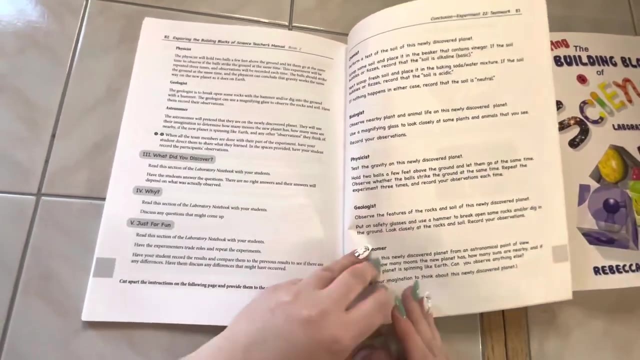 sad little complaint is that i wish they could somehow combine this book you with the lab notebook, because it's kind of bulky and frustrating to try to go back and forth between the two because you do need both of them to do the experiments. i wish there was a way they could. 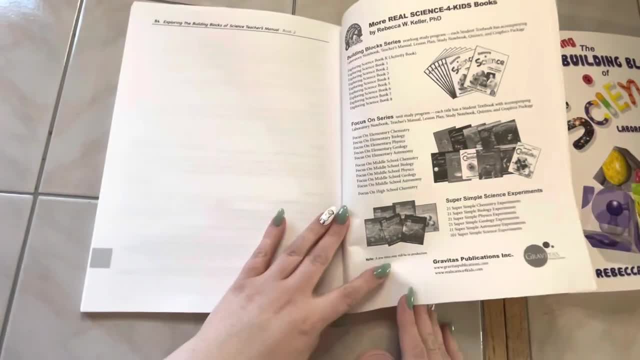 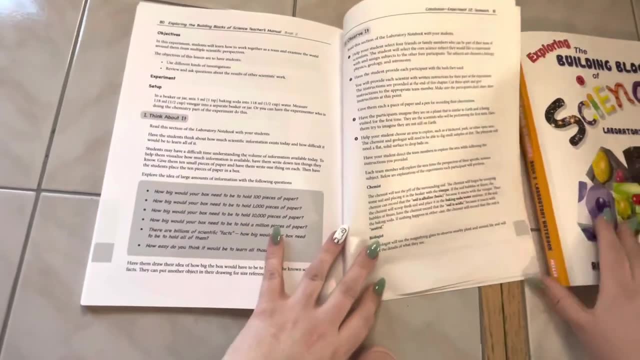 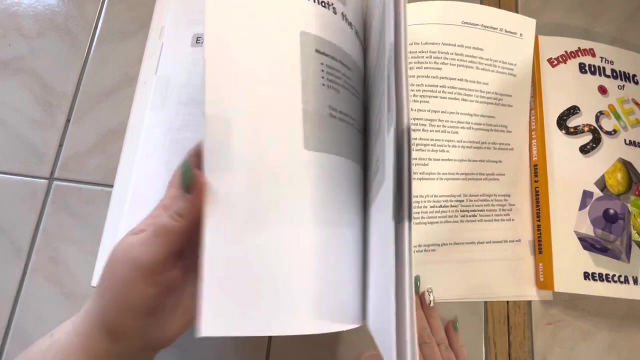 combine the two books and make it easier for. but i think they also use these in schools, which is probably why it's broke out like this, because then you can hand each student their lab notebook or printed off copies, and then the teacher has their book to tell the kid what to do, or children. 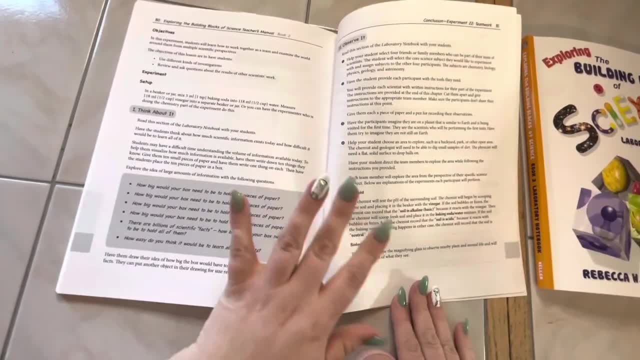 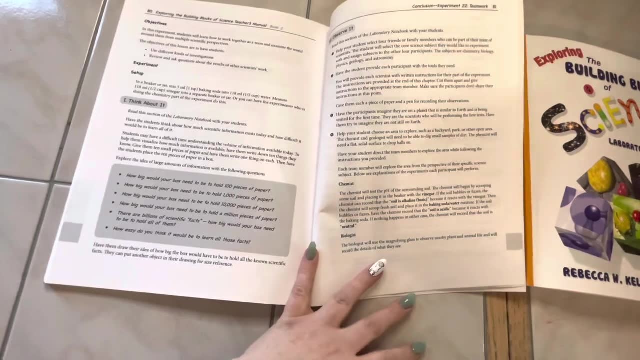 what to do. but, as i said, i wish they could combine the two books and make it easier for them to do. as a homeschooler, i would much prefer these two books to be combined in a way and make it less bulky and less books, or even combine all three books somehow, making it even less bulky for me. 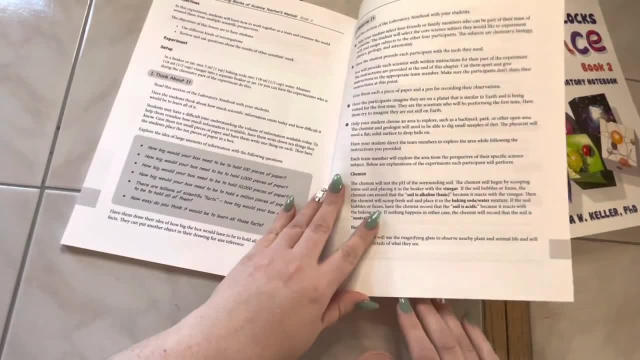 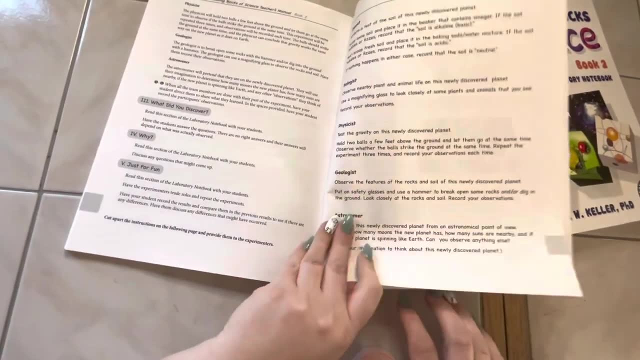 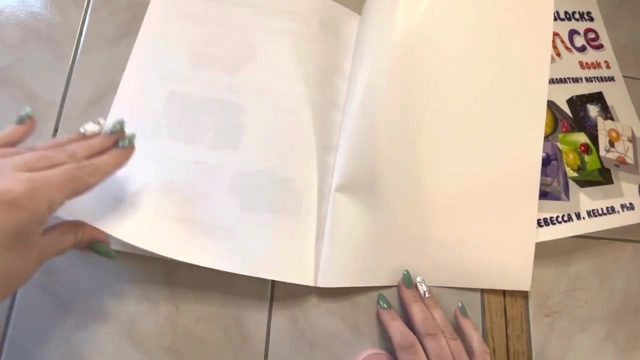 and that would be preferred than trying to have to keep track of three books. or when we're doing experiments, i have to keep two books open, which is my only, my only downside at all to this entire curriculum. I love this curriculum. I think it's engaging, it's fun and it has all the information. 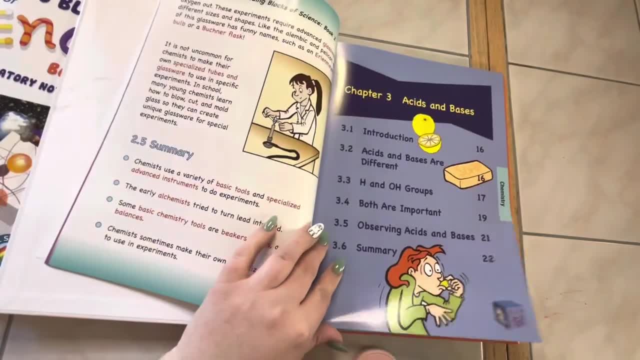 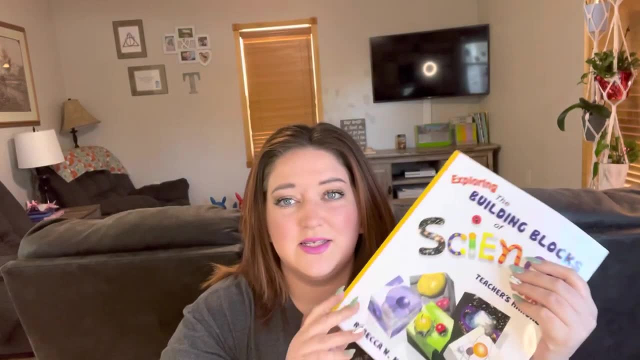 that I want my child to learn about science. I enjoy the book. I think it's fun engaging. my children love it. Okay, so that was everything in the building blocks of science as a down shot, so you can see through the pages and look at them yourself. If you have any questions for me, please, 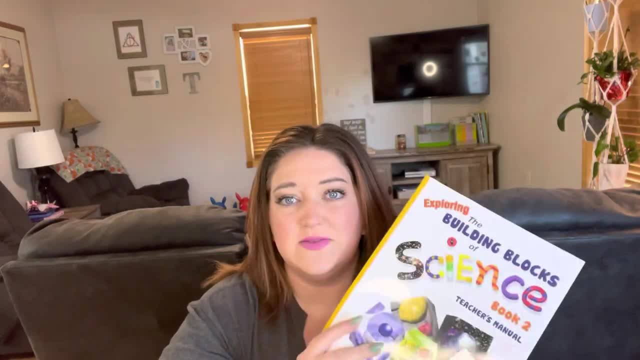 leave them in the comments below. I will leave a link to building blocks of science and timber doodle below as well, and I really appreciate you watching. Thank you so much. I'll talk to you next time.